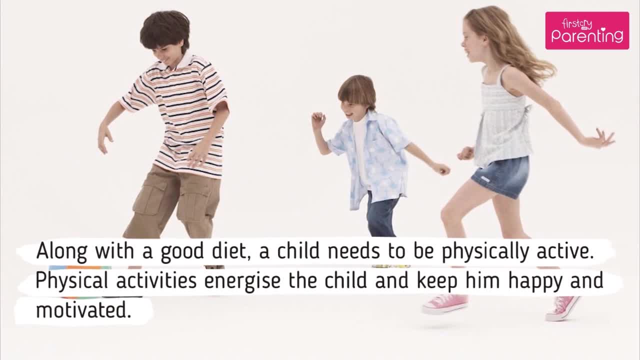 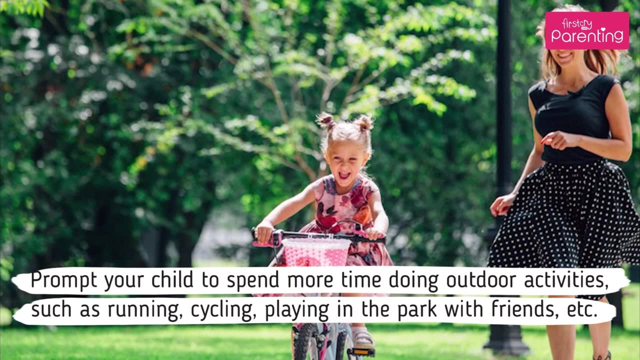 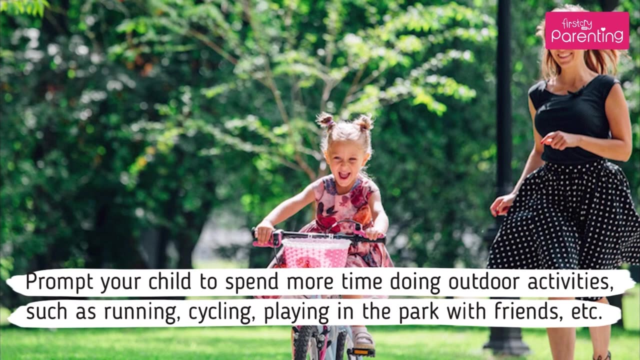 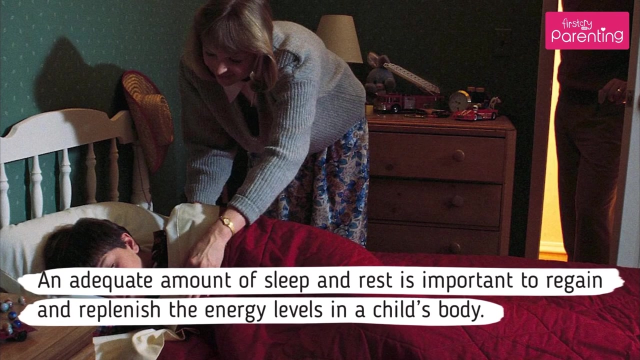 and diet. A child needs to be physically active. Physical activities energize the child and keep him happy and motivated. Prompt your child to spend more time doing outdoor activities such as running, cycling, playing in the park with friends, etc. 3. Sleeping on time: An adequate amount of sleep and rest is important to regain and 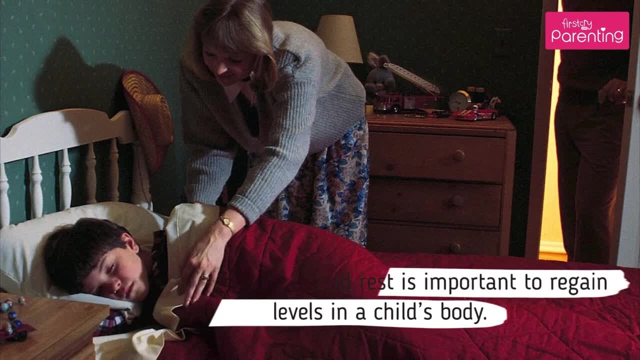 replenish the energy levels in a child's body. 1. Sleep and rest. Sleep and rest are important to regain and replenish the energy levels in a child's body. Set a sleeping routine for your child and adhere to it. Irregular sleeping. 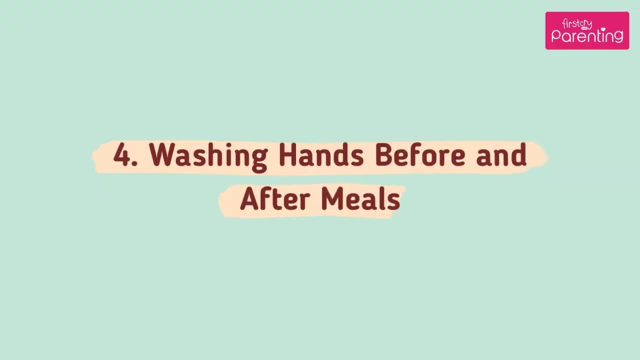 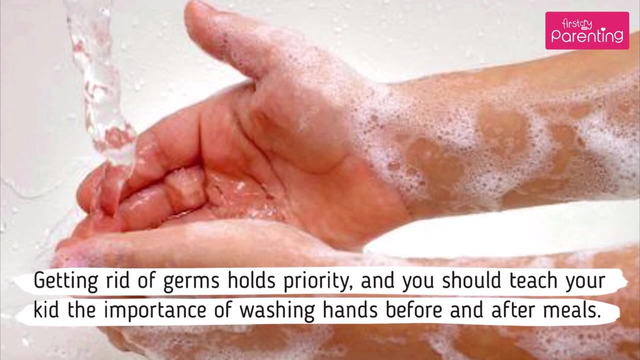 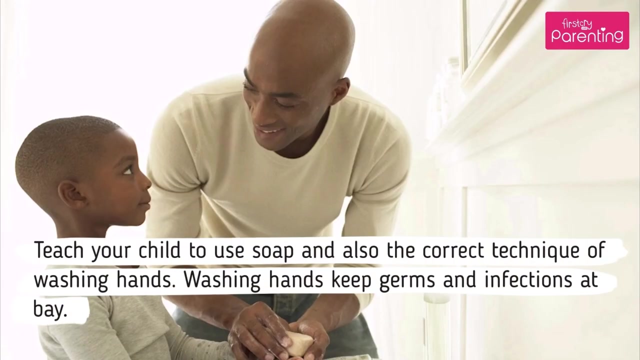 hours can make him irritable and erratic. 4. Washing hands before and after meals. Getting rid of germs holds priority and you should teach your kid the importance of washing hands before and after meals. Teach your child to use soap and also the correct technique of washing hands. Washing hands keep germs. 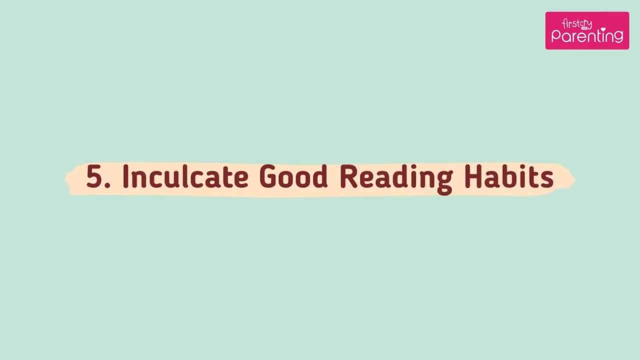 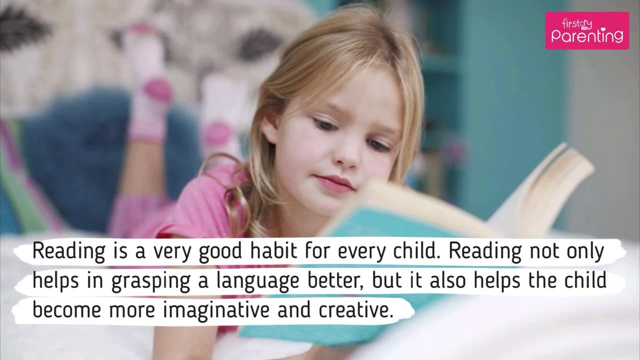 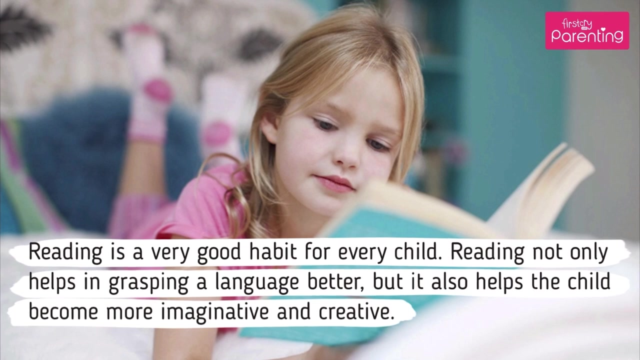 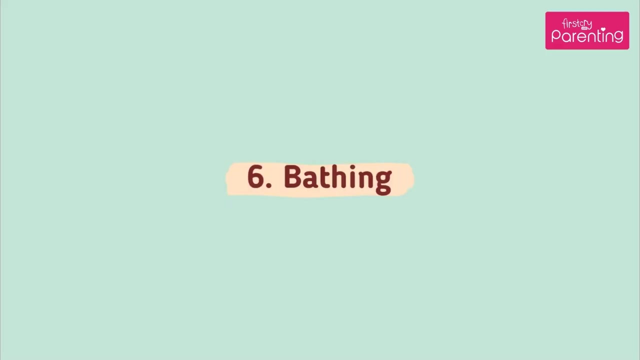 and infections at bay. 5. Inculcate good reading habits. Reading is a very good habit for every child. Reading not only helps in grasping a language better, but it also helps the child become more imaginative and creative. You may set up a regular reading schedule or even read together at bedtime. 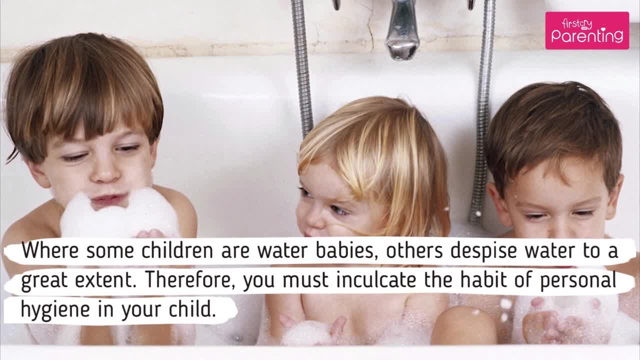 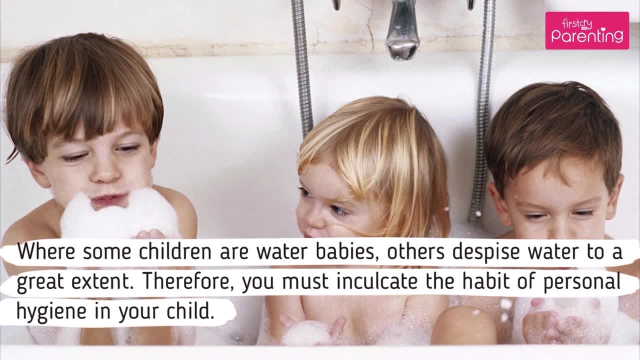 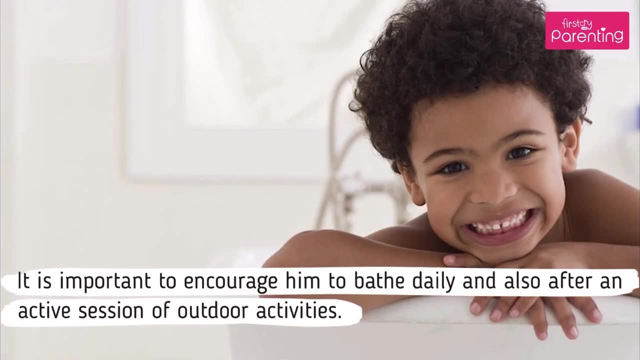 6. Bathing. Where some children are water babies, others despise water to a great extent. Therefore, you must inculcate the habit of personal hygiene in your child. It is important to encourage him to bathe daily and also after an active 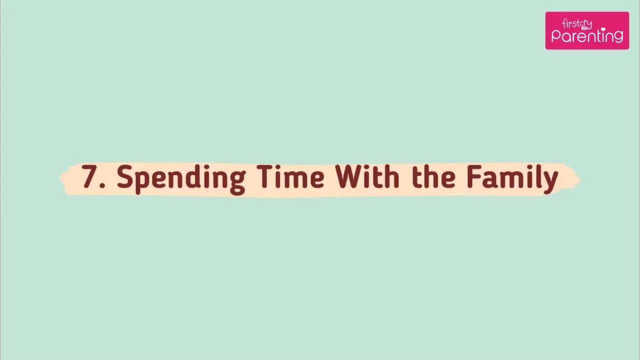 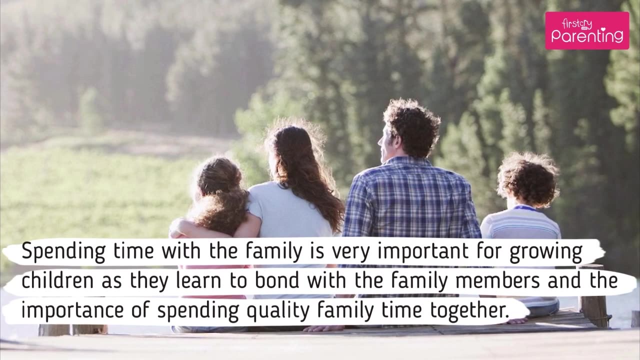 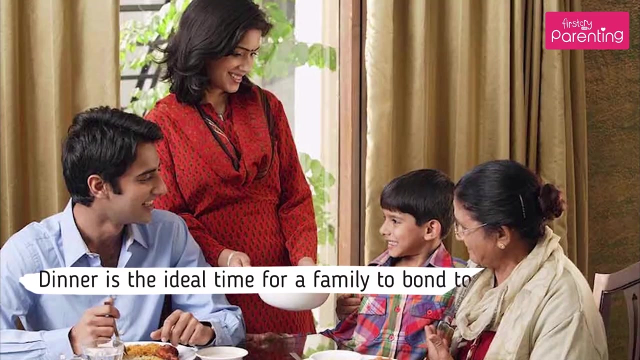 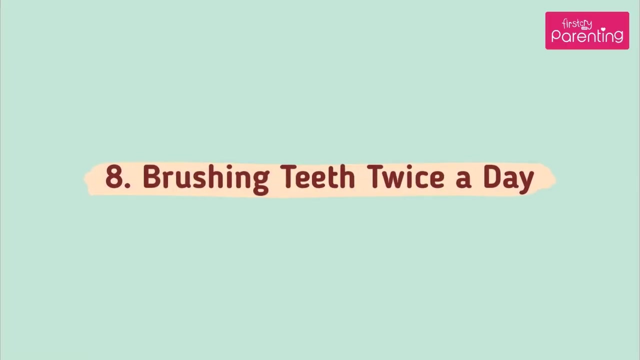 session of outdoor activities. 7. Spending time with the family. Spending time with the family is very important for growing children as they learn to bond with the family members and the importance of spending quality family time together. 8. Brushing teeth twice a day. You should strictly help your child follow the habit. 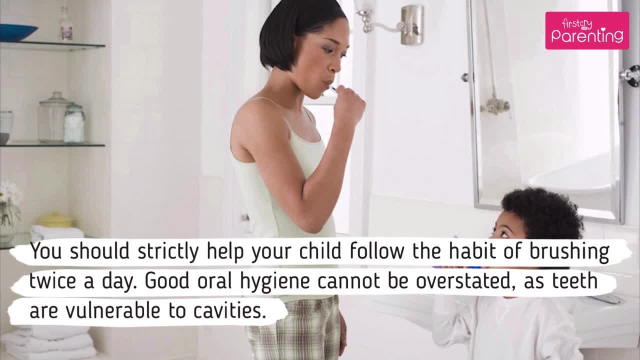 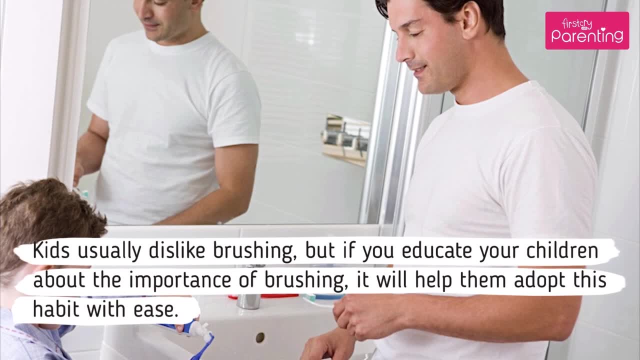 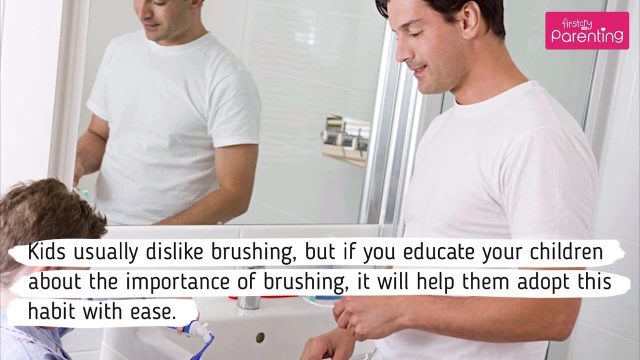 of brushing twice a day. Good oral hygiene cannot be overstated, as teeth are vulnerable to cavities. Kids usually dislike brushing, but if you educate your children about the importance of brushing, it will help them adopt this habit with ease. 7. Brushing teeth. Brushing teeth is a very important habit for children. It is important. 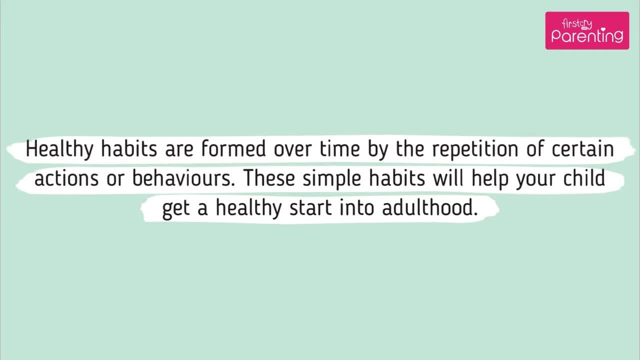 for them to brush their teeth regularly. 8. Brushing teeth: Brushing teeth is a very important habit for children. It is important for them to brush their teeth regularly. Kids usually dislike brushing, but if you educate your children about the importance of brushing, it will help them adopt this habit with ease. 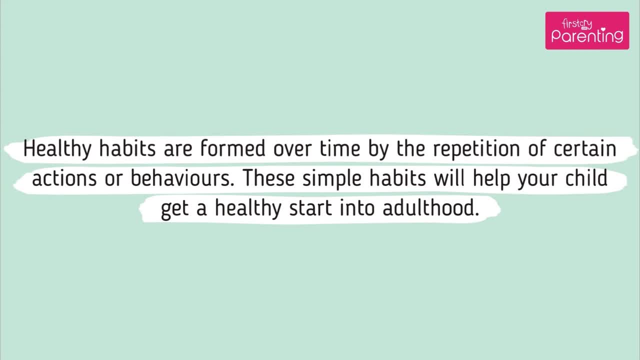 Healthy habits are formed over time by the repetition of certain actions or behaviors. These simple habits will help your child get a healthy start into adulthood. 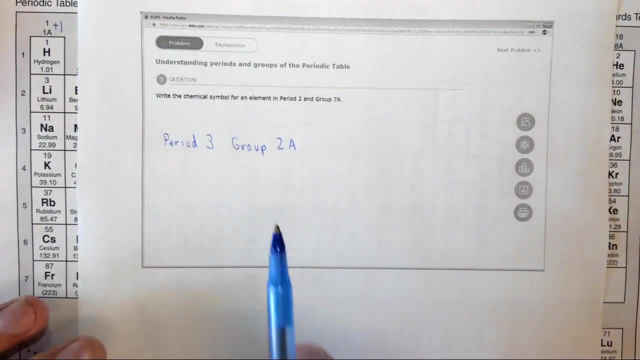 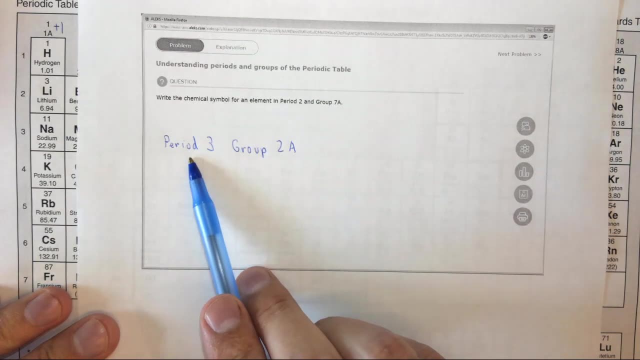 In this question we're asked to write the chemical symbol of an element in period 2 and group 7a of the periodic table And as another example we're also going to find period 3 and group 2a. So the periodic table is arranged in. 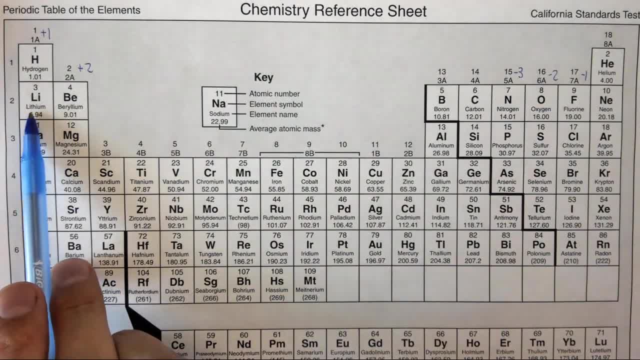 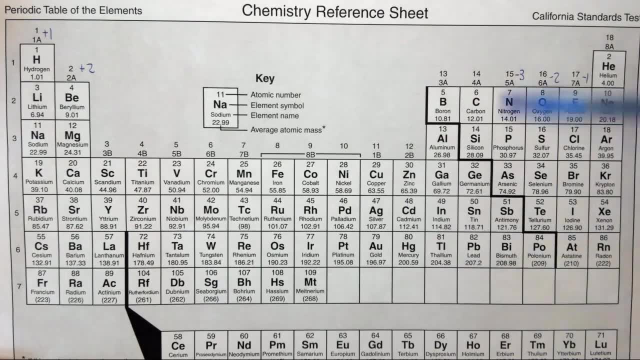 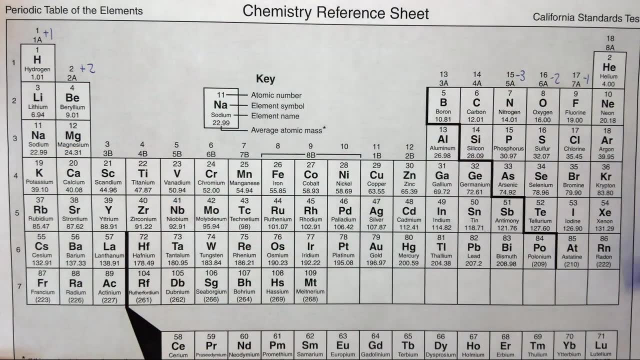 periods, which are your horizontal rows on the periodic table, and groups, which are your vertical columns on the periodic table. You may recall from the class that elements in the same group have similar chemical properties. So the noble gases, for example, have similar chemical properties in group 8a or 18,. 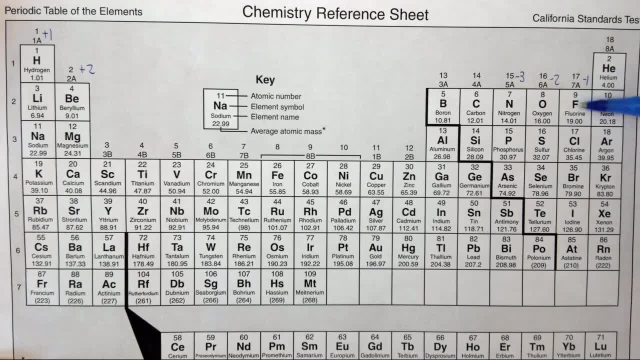 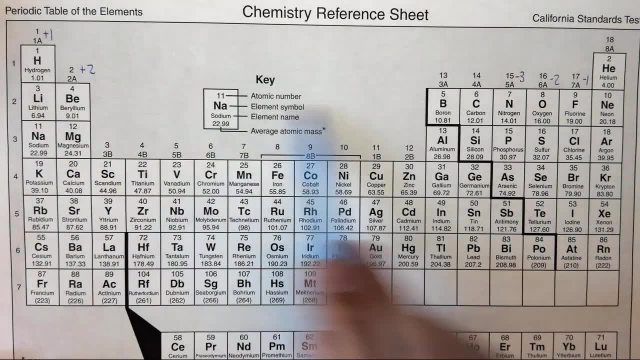 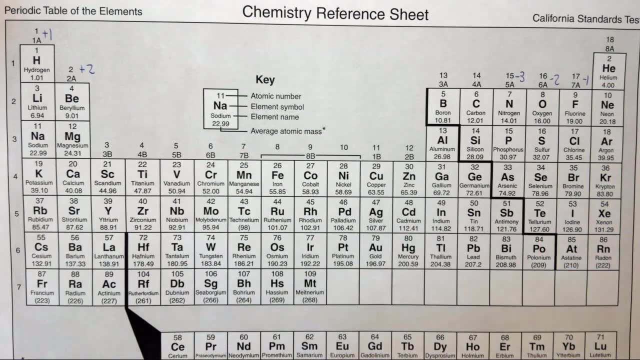 and or halogens in group 7a or 17 have similar chemical properties to each other. However, for this question, all we need to know is that the periods are the horizontal rows and the groups are the vertical columns. So, going back to the original question, period 2,. 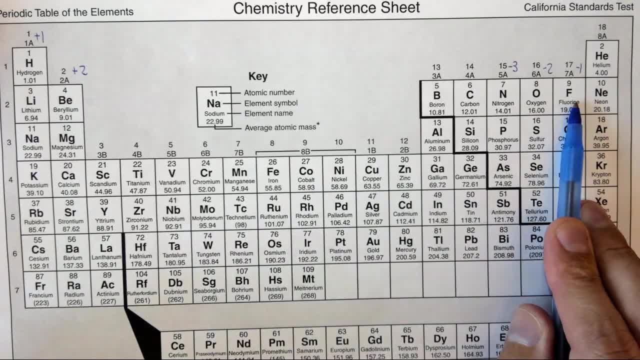 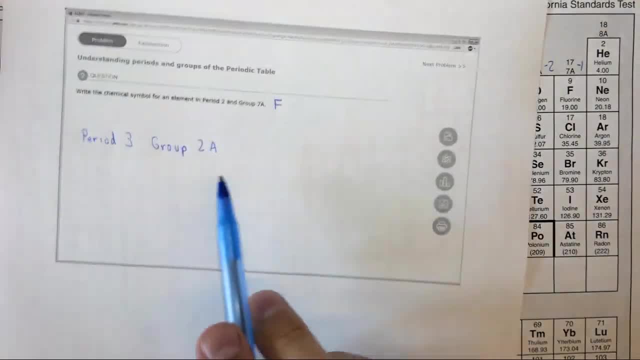 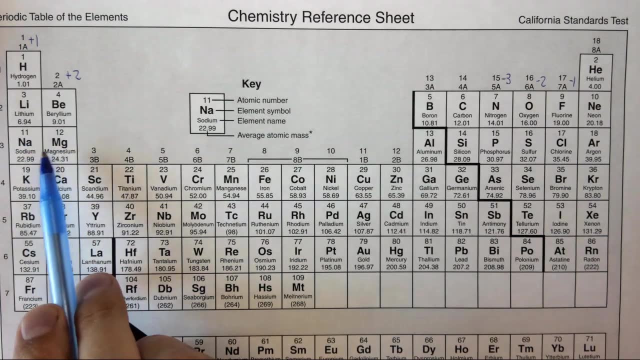 group 7a. period 2, group 7a. it's a halogen, it's fluorine, Also, as my other example, period 3, group 2a. So period 3, group 2a, which is an alkali earth metal. 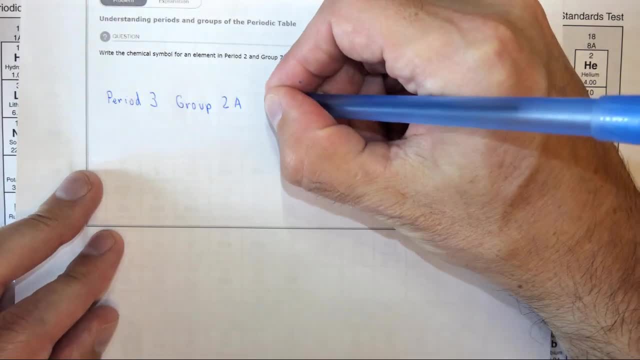 which is magnesium. Thank you.